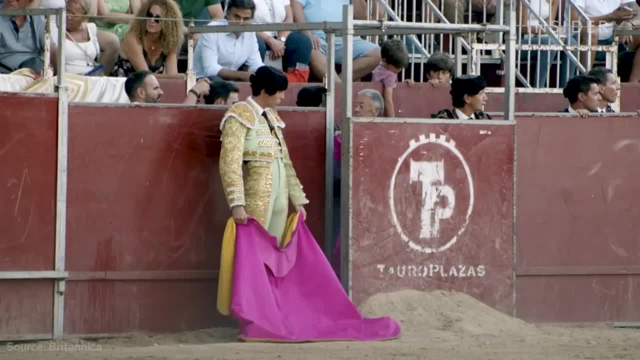 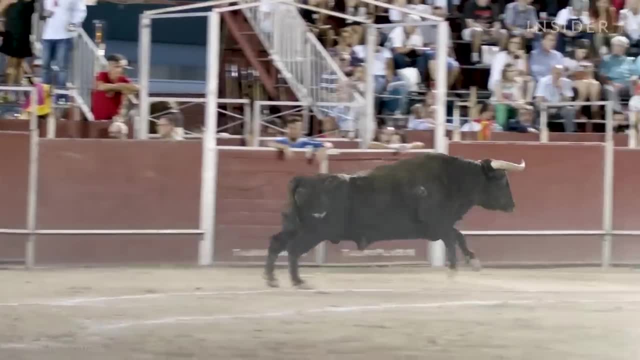 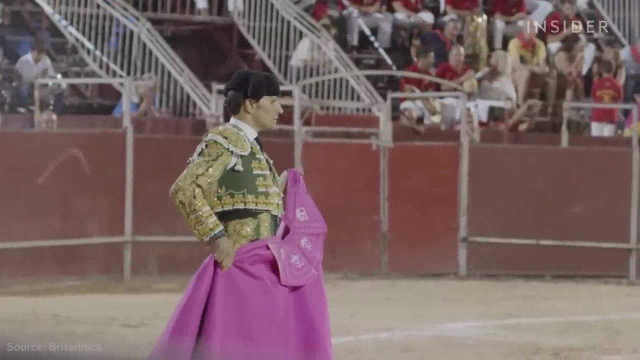 And the pitbull is taken by about half a dozen bullfighters. The bulls are kept in a small dark pen for hours before the fight so they'll chase the light and storm into the arena. once the gates open They will take turns facing the bull, feeling his temperament and tiring him out. 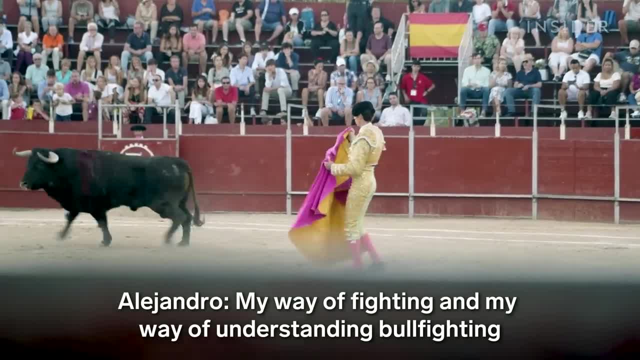 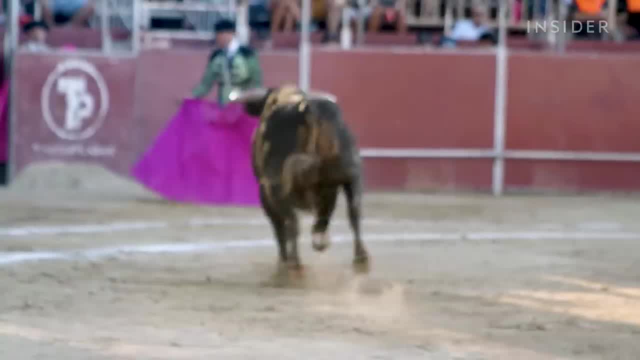 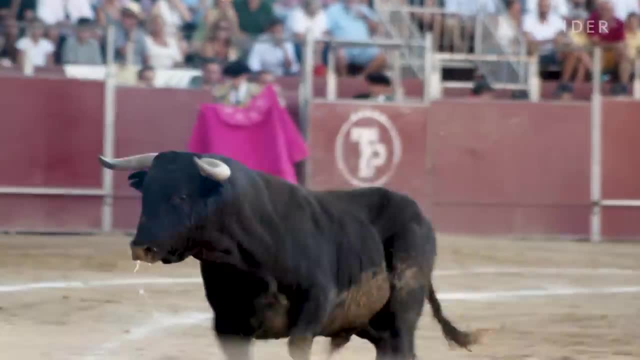 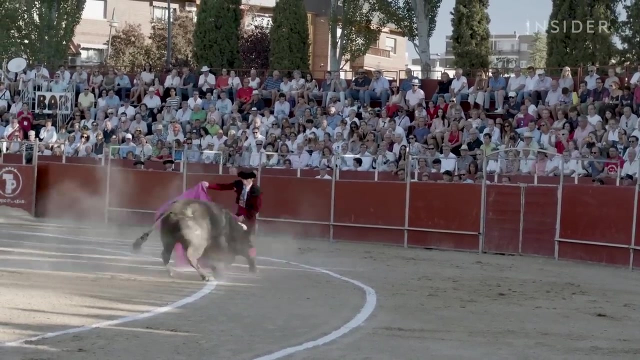 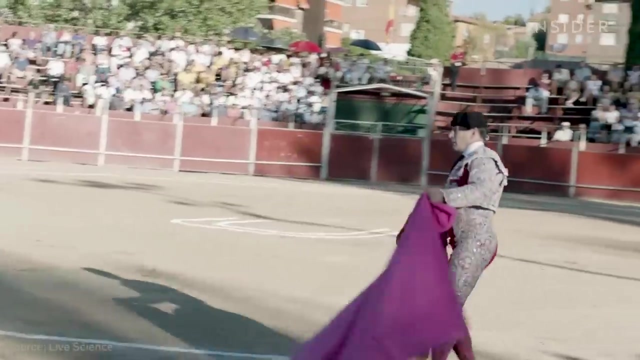 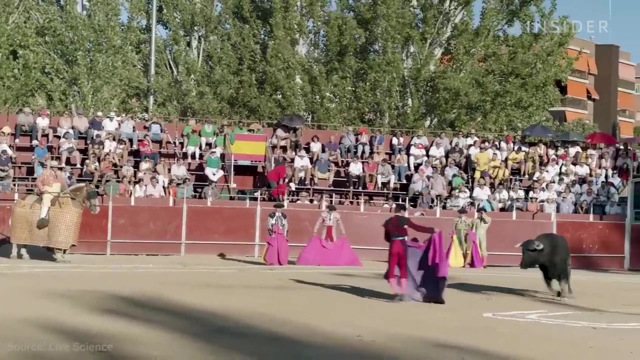 He screams for a song about to Hephaestus. From my way of networking and understanding networking, I like to see him less often so that we can create something artistic, beautiful and that people don't forget The movement of the cloak is what triggers them. 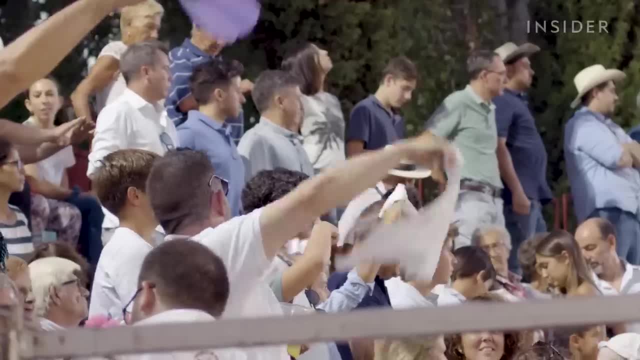 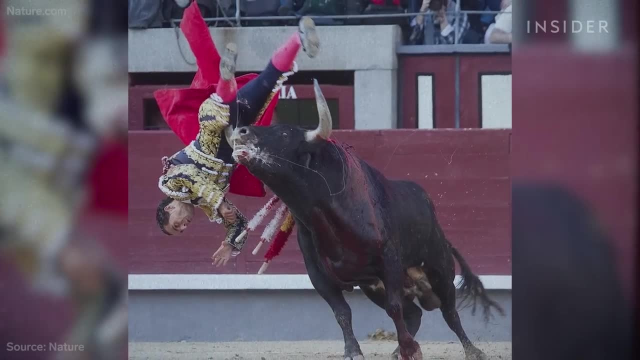 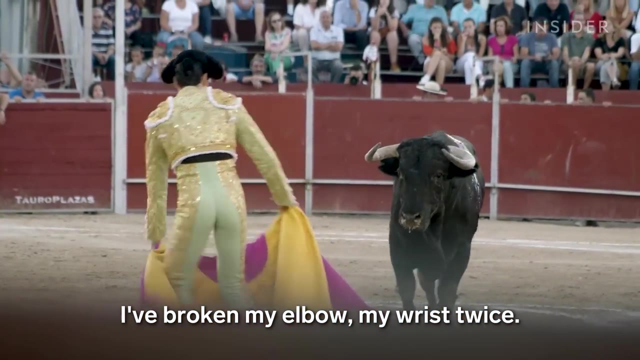 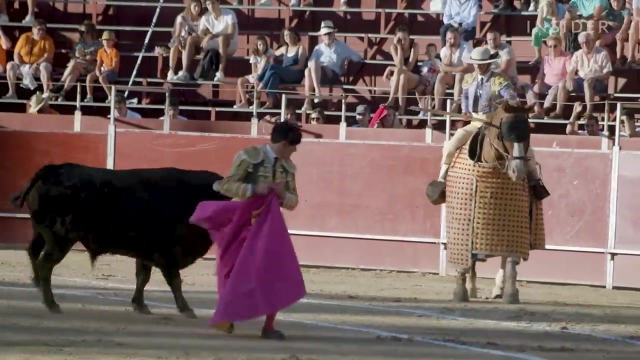 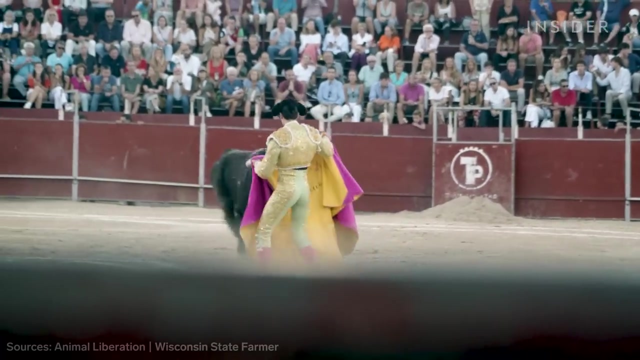 Alejandro has to be quick on his feet to avoid any injuries. There's about one accident for every ten fights. The most common are gorings. In the end it's an unpredictable animal. Bulls are not natural predators, they're prey. That's why they're fearful and reactive and charge only when provoked. 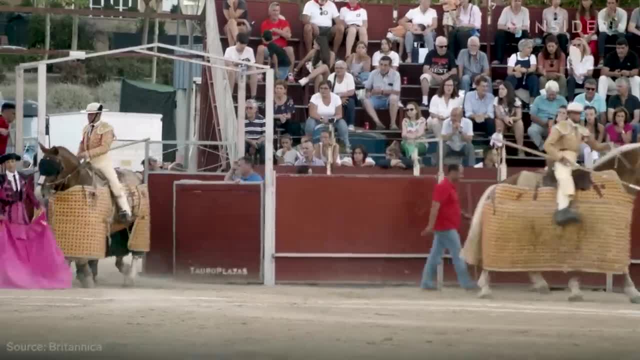 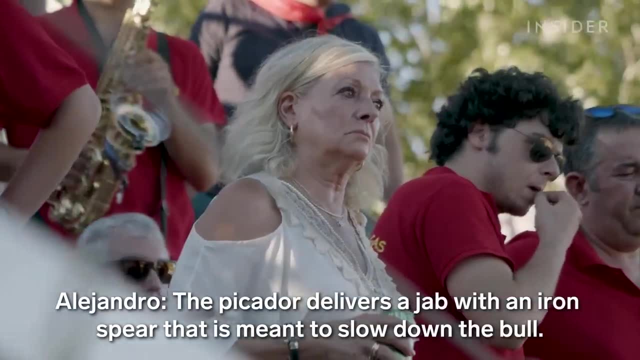 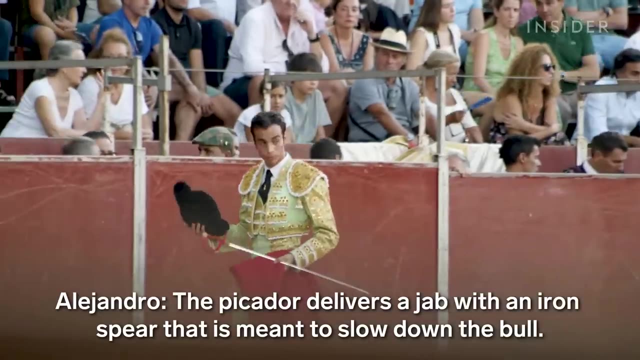 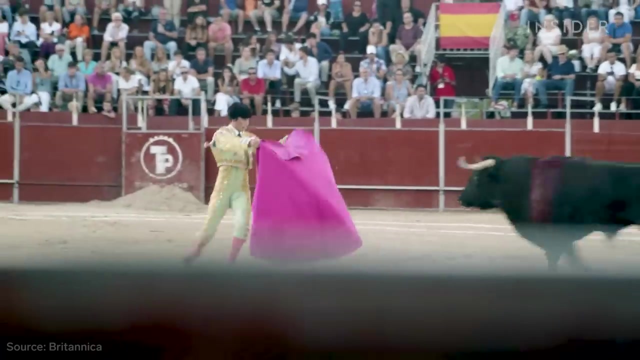 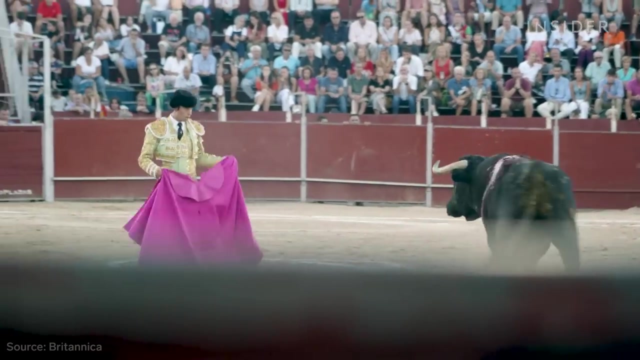 Toward the end of Act One, bullfighters on horseback, called picadors, enter the ring and stab the bull with spears. After that, Alejandro attracts the bull's attention away from the picadors with cape passes performed like a dance. 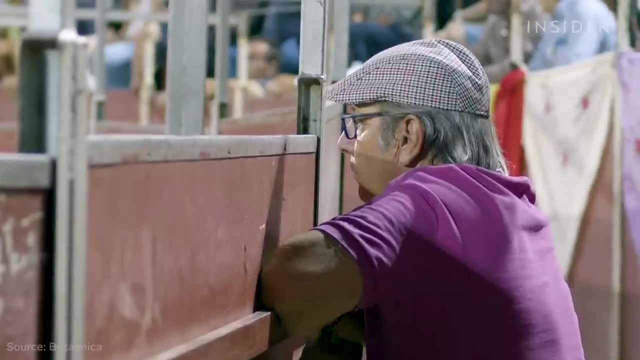 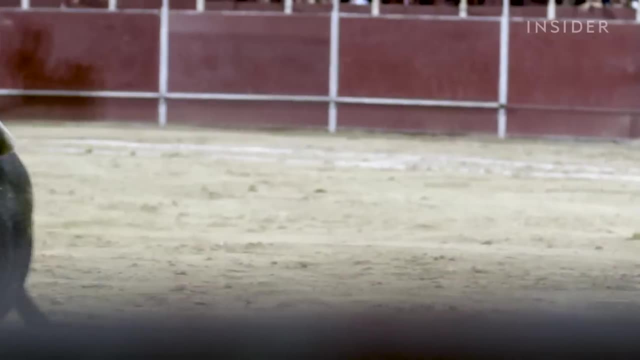 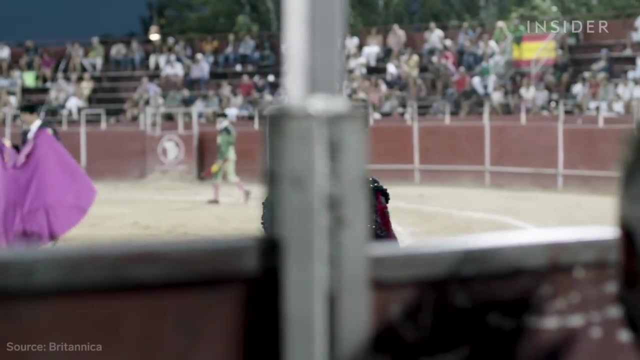 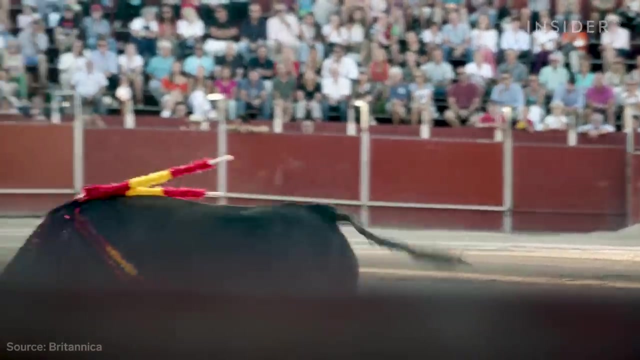 The bullfighters eventually leave the ring to take a break, But the bull stays. Act Two is one of the most controversial parts. The bullfighters re-enter the ring, taking turns, stabbing the bull between its shoulders with these sharp darts called banderillas. 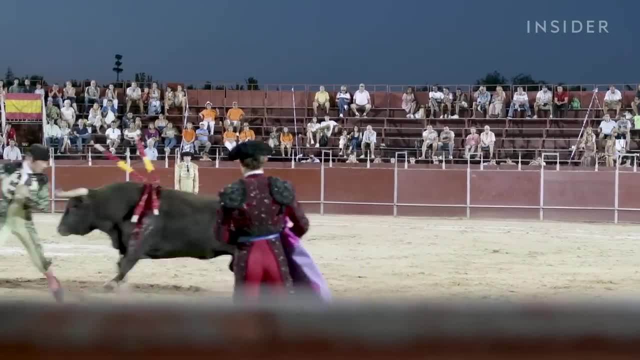 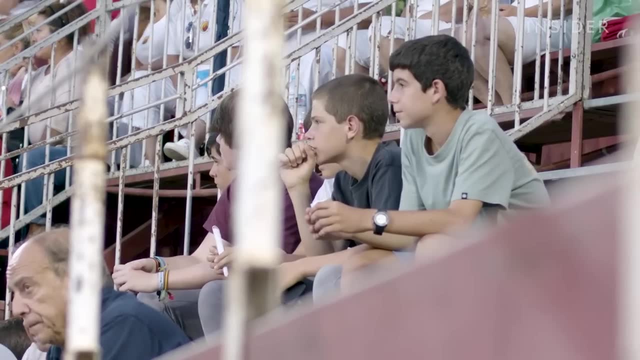 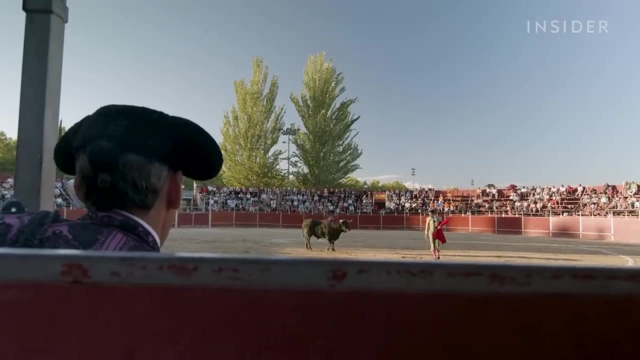 This goes on for about 15 minutes. If this video is hard for you to watch, you're not alone. There are countless petitions to end bullfighting all over the world, And the art has been the center of controversy for decades. Historians have long debated the exact roots of bullfighting. 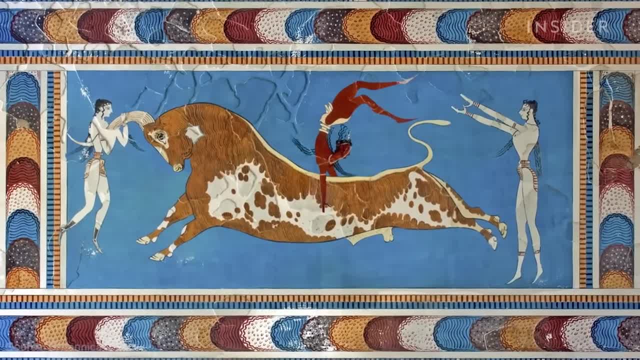 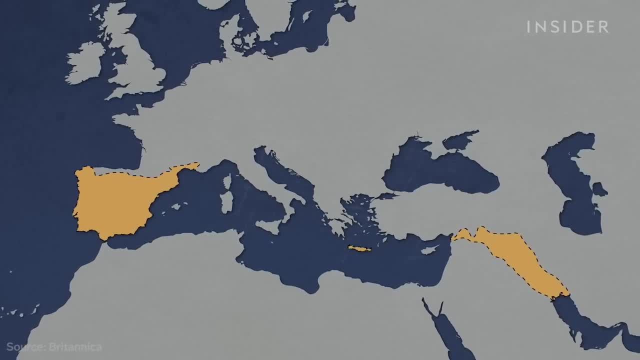 but they know versions of it existed as early as 1500 BCE and were popular across Mesopotamia, Moorish Spain, the Greek island of Crete and ancient Rome, where gladiators fought bulls in the Colosseum. 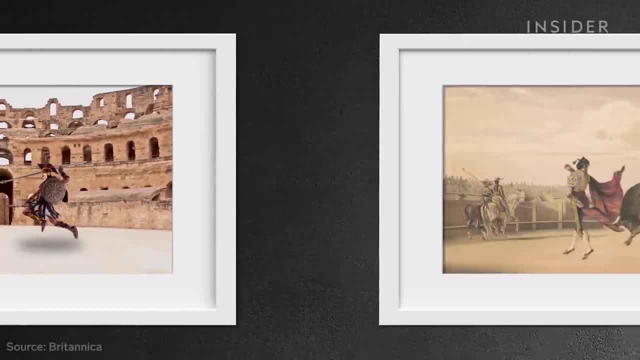 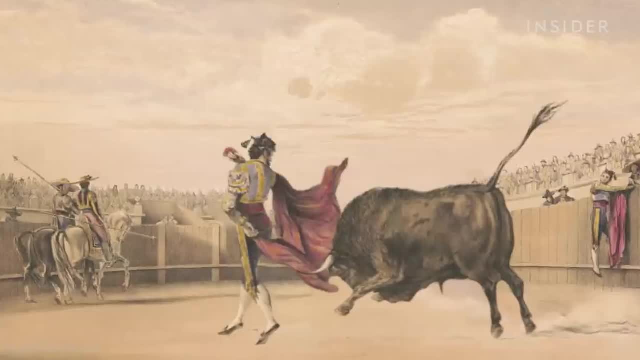 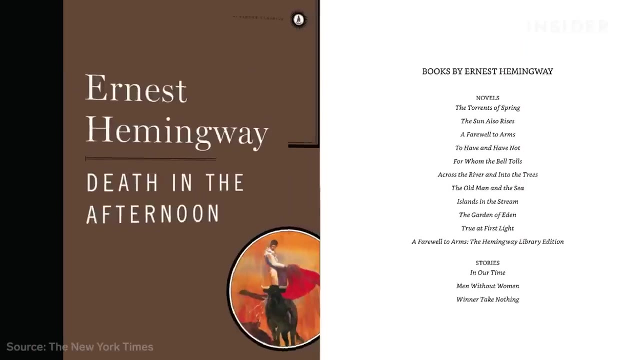 The bull represented power and fertility, and that became part of a popular spectacle in Spain in the 1500s, the matador portraying masculinity by killing a bull. Its appeal continued into the 20th century. In 1932, Ernest Hemingway wrote: 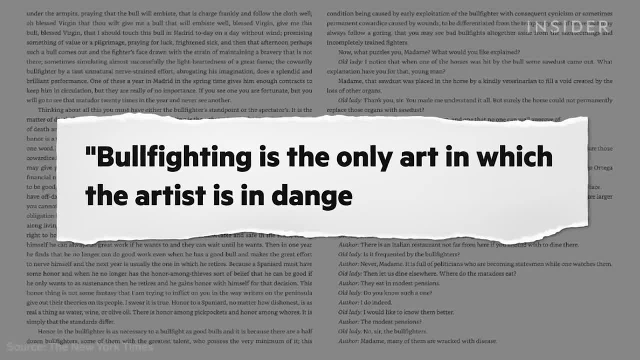 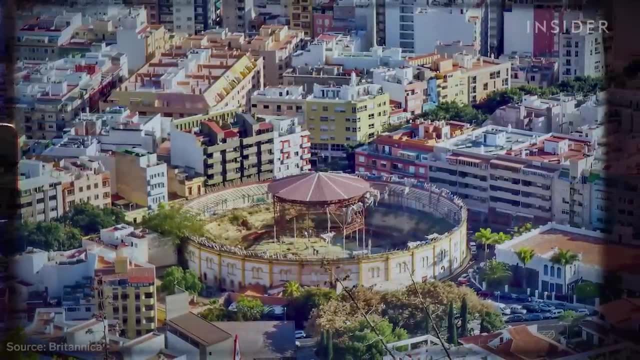 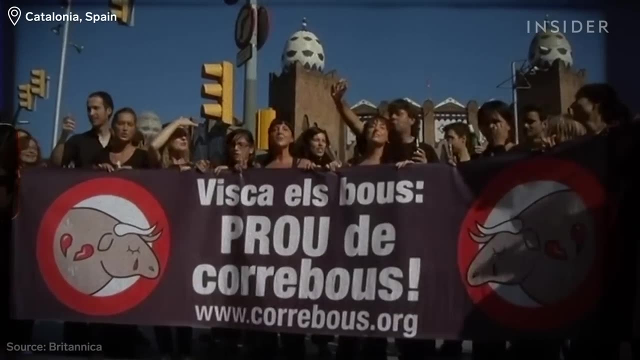 Bullfighting is the only art in which the artist is in danger of death. Toward the end of the 1900s, however, bullfighting fell out of fashion. Spain's Canary Islands banned it in 1991.. And in 2010,, Catalonia blocked it as well. 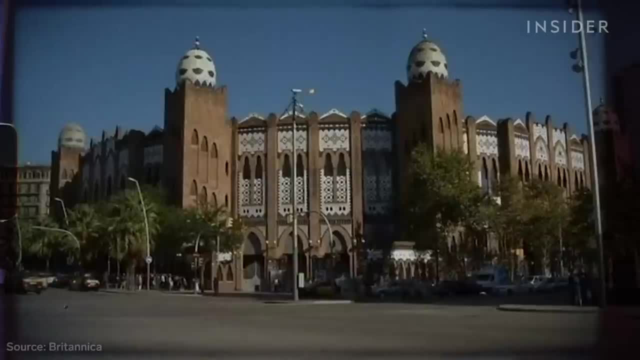 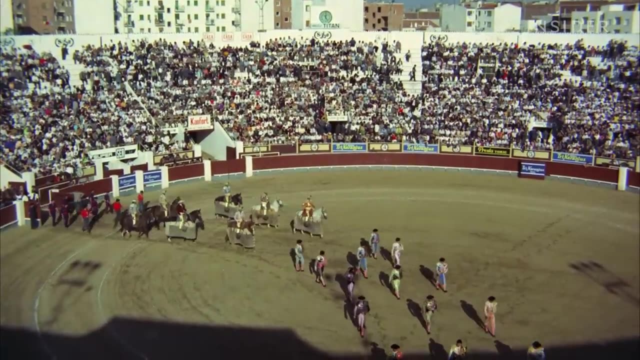 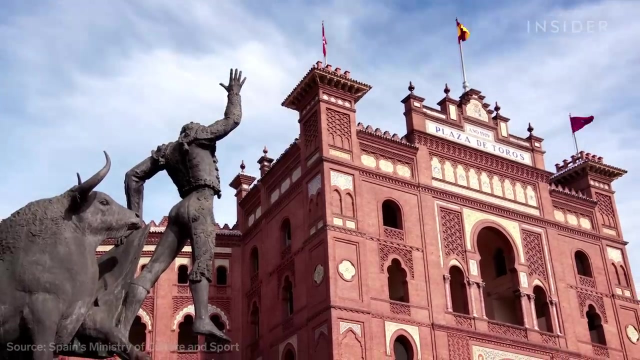 This was a big deal because the region's capital, Barcelona, has a long bullfighting history. And then the pandemic hit. There were about 1,500 bullfights a year in Spain before COVID-19.. But now there are fewer than 900. 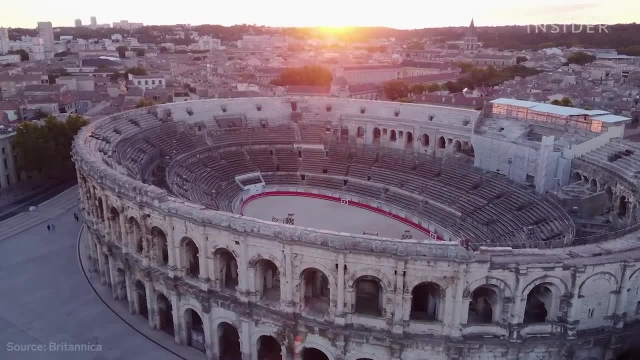 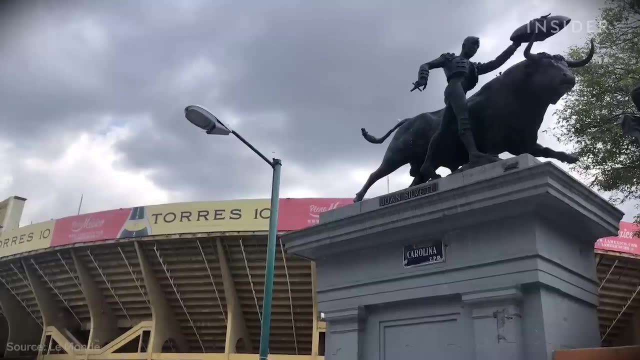 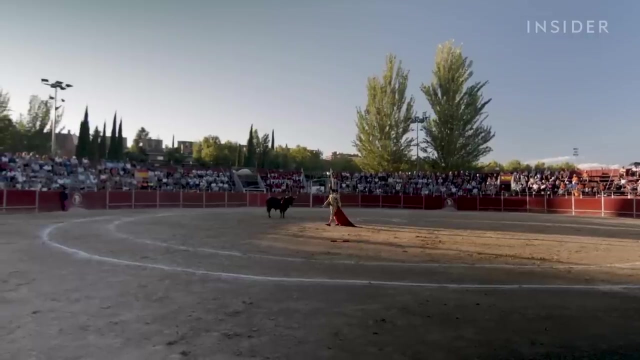 The practice is also declining across the world. The largest ring in the world now sits empty in Mexico City after a court banned bullfighting there in June 2022.. Animal rights activists say this is a cruel and outdated tradition in which the bull is tormented. 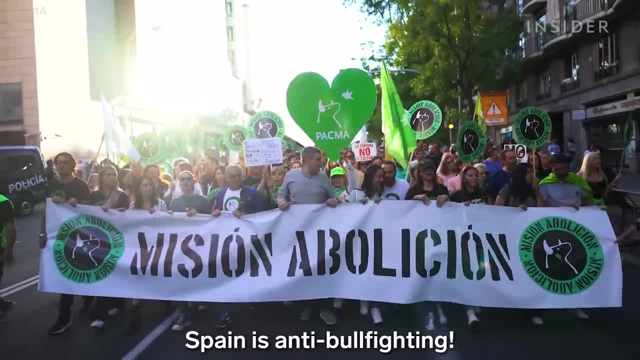 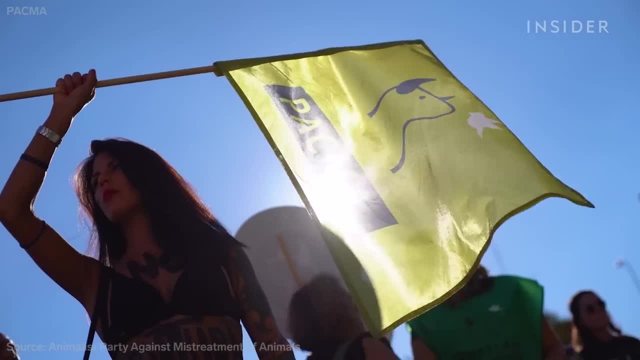 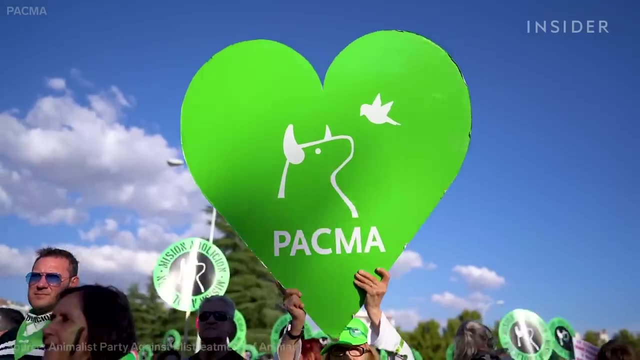 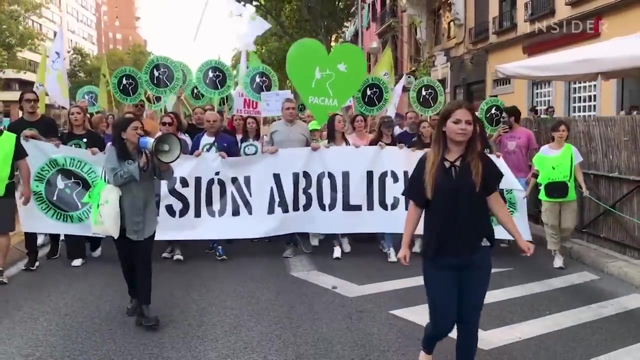 It is anti-bullfighting. Spain is anti-bullfighting. In September, 5,000 people showed up to a protest in Madrid organized by the Animalist Party Against Mistreatment of Animals, or PACMA. Ana Bejar volunteers with PACMA. 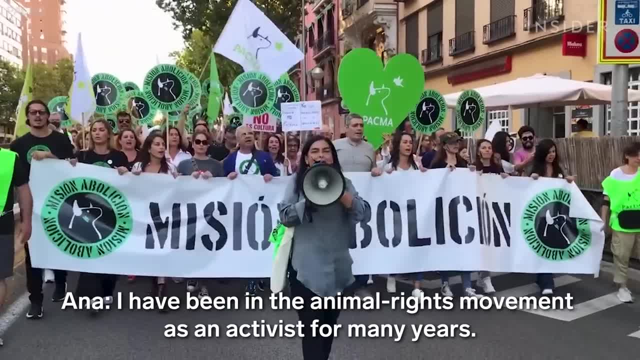 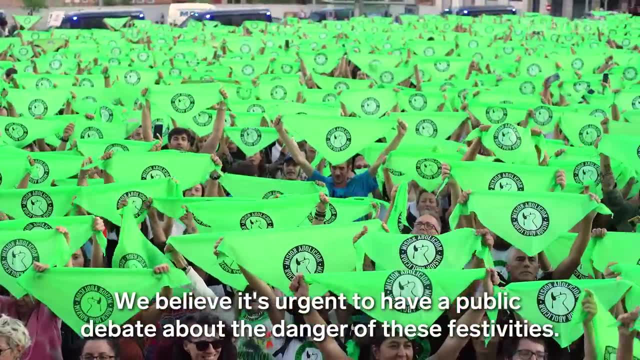 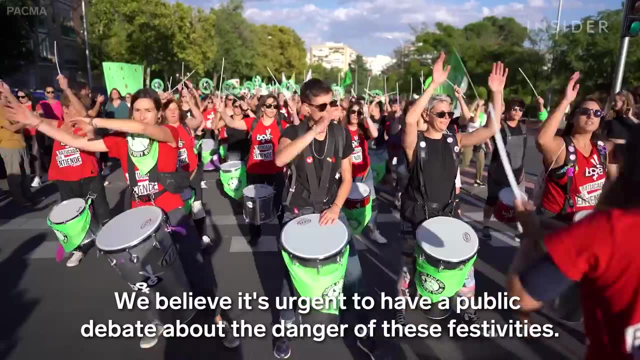 I've been in the animal movement as an activist for many years. I've been a vegan for 15 years. Mission Abolition, Mission Abolition. We believe that it is urgent that we stand at the table, that we socially debate the danger of this kind of celebration. 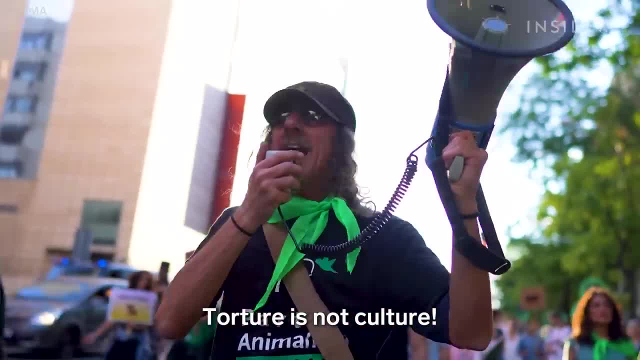 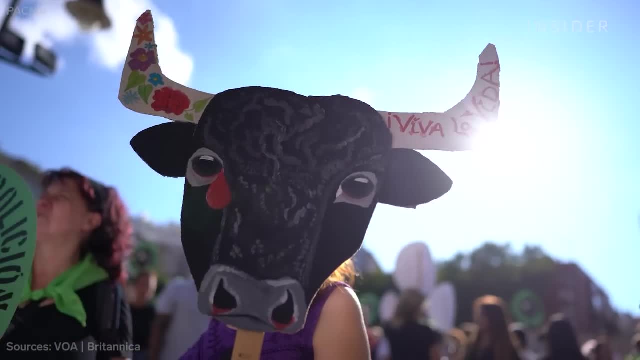 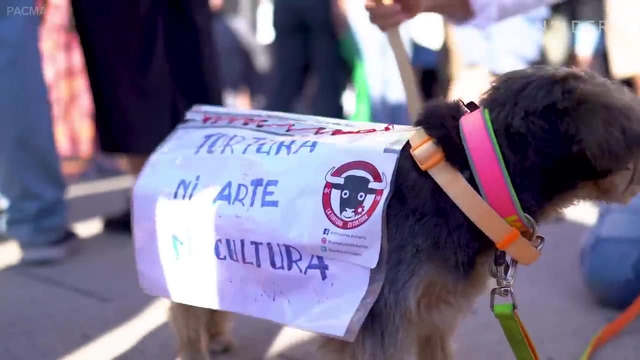 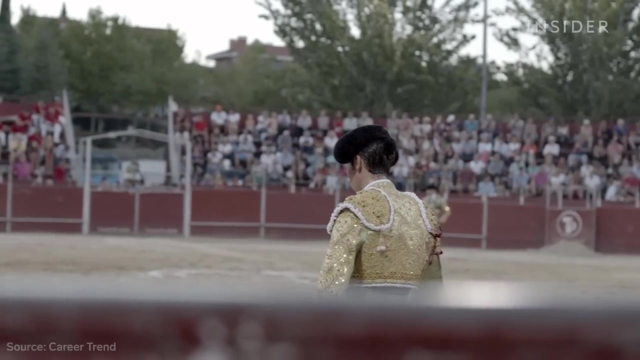 Torture is not culture. Still in Spain, the fights bring billions of euros to the Spanish economy and employ an estimated 200,000 people. We are going to close this square. Matadors like Alejandro can make up to $150,000 per year. 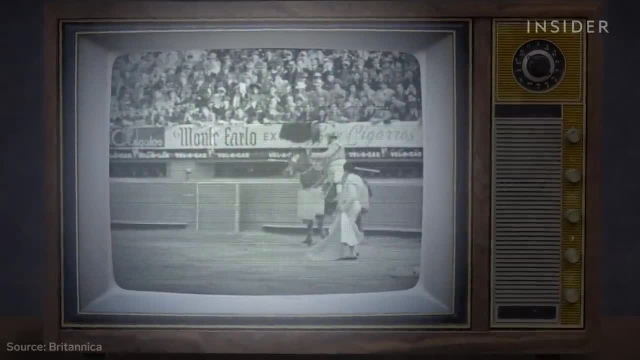 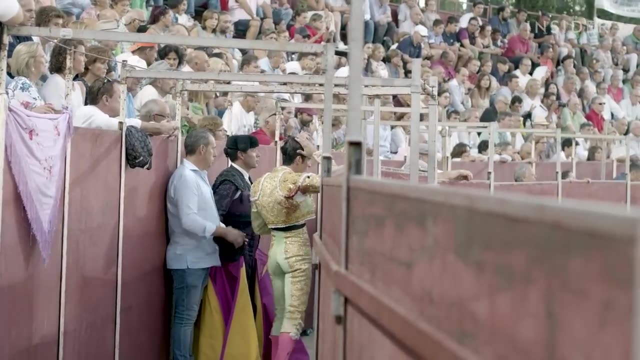 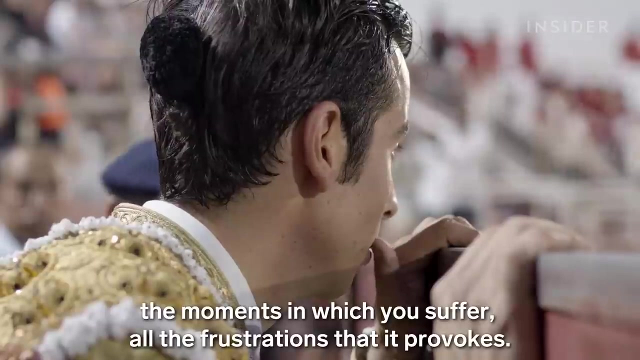 Nowadays, bullfighters associate the practice with freedom of expression and Spanish identity. Still, Alejandro doesn't want his son to follow in his footsteps. There are many things that this entails: The tastelessness that it leaves you, the moments in which you suffer. 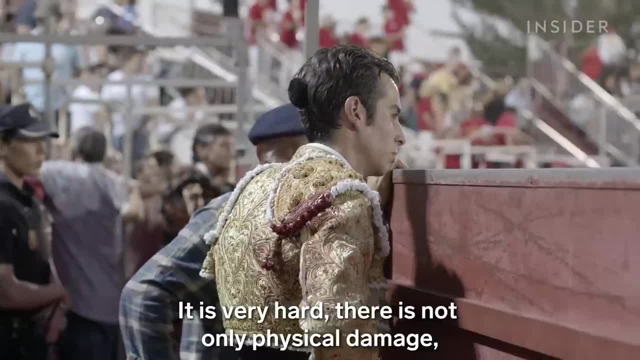 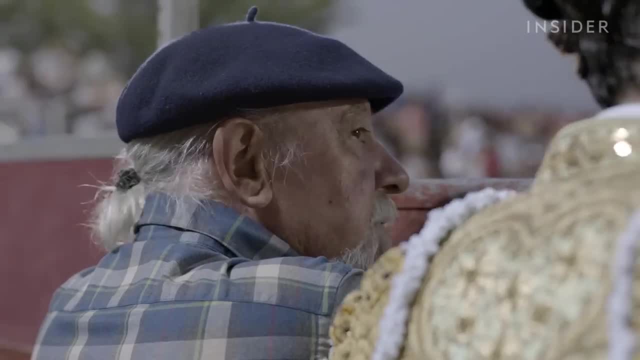 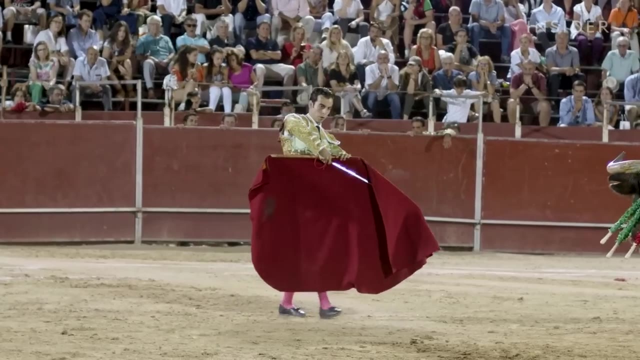 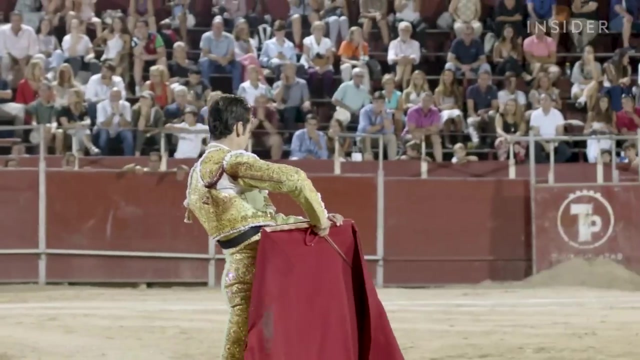 the frustrations that it can cause you. There are very hard moments, not only physical but also mental, that are difficult to overcome. Back in the ring, Alejandro faces the bull with a sword in hand. He uses the iconic red cape called the muleta. 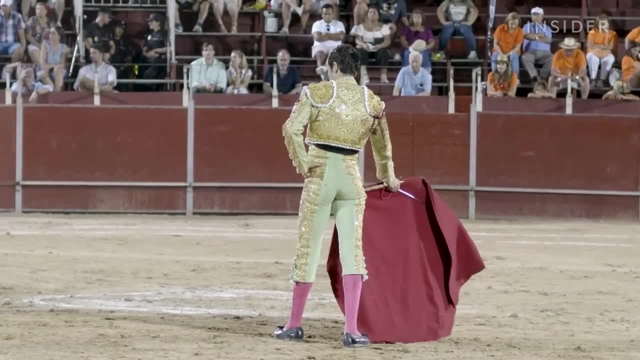 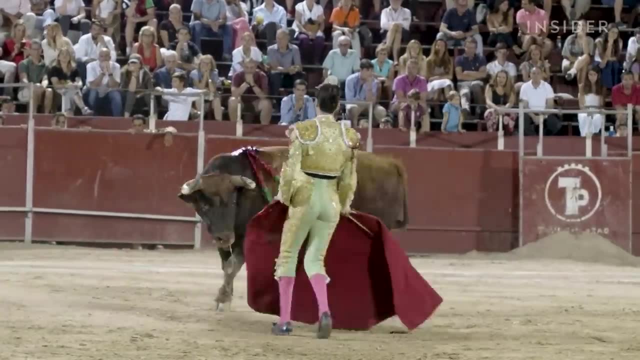 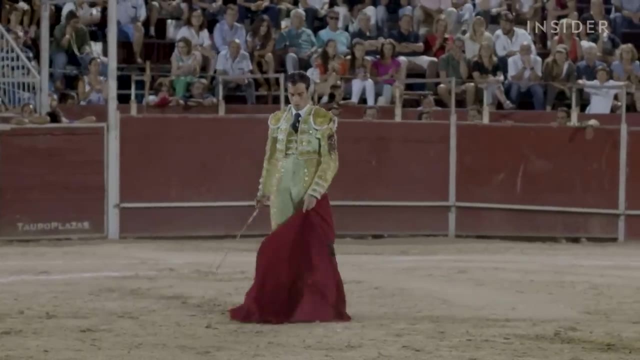 to attract the bull. in another series of passes Demonstrating his control over the animal, matadors use red to hide the bull's blood. We weren't allowed to film act three, when the bull is killed. I also like animals, like everyone else. 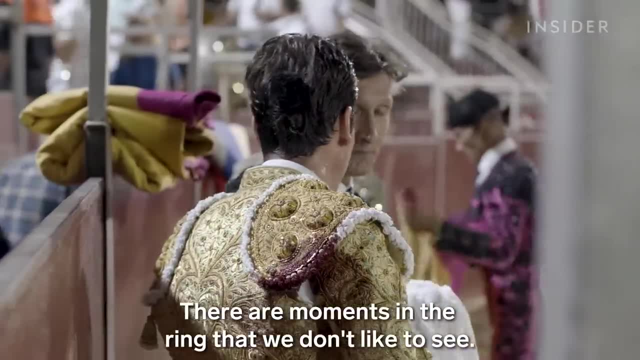 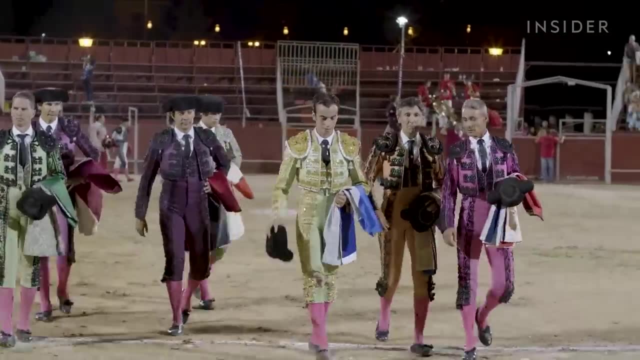 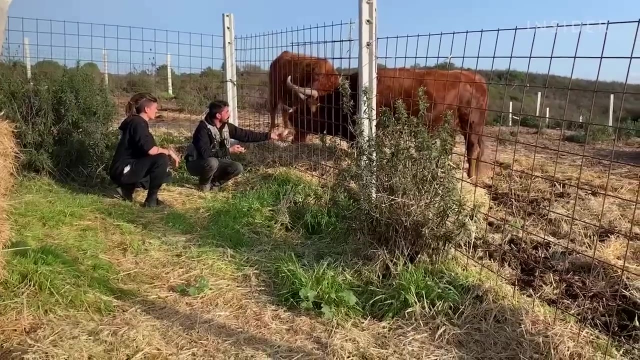 but there are moments in the square that we don't like to see. The meat is processed at a slaughterhouse and then distributed to vendors. Rescuing a bull from a ring is nearly impossible- The animals that are used during bullfights. 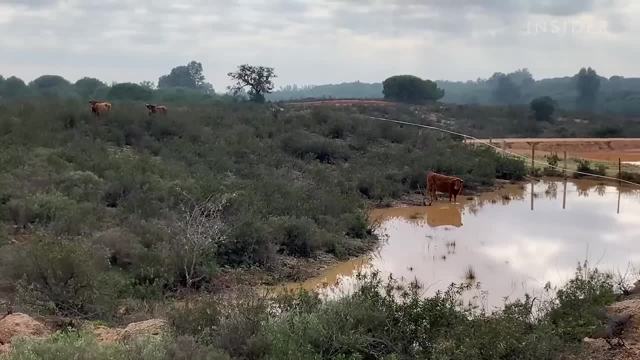 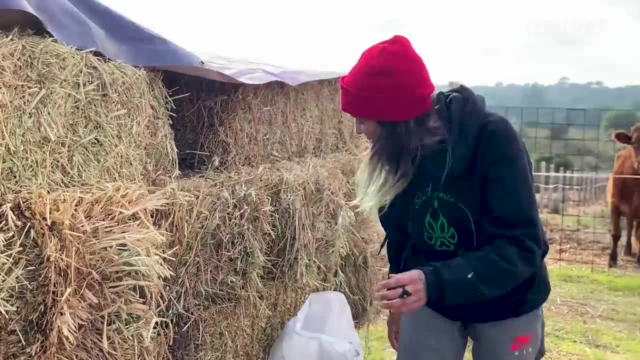 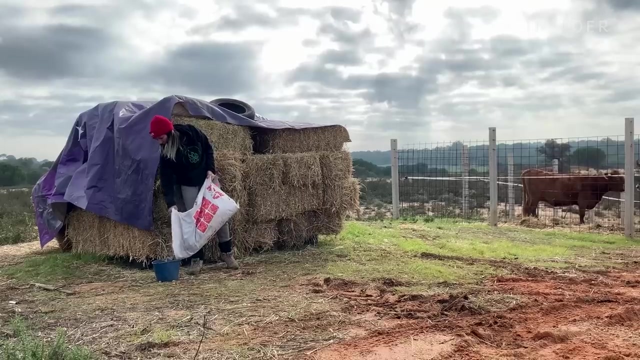 they die in the bullfight, so they cannot be rescued. Maite van Gerwen is the director of CAS International, an NGO based in the Netherlands that has rescued bulls since 2016.. They buy them from breeders before they ever enter a fight.